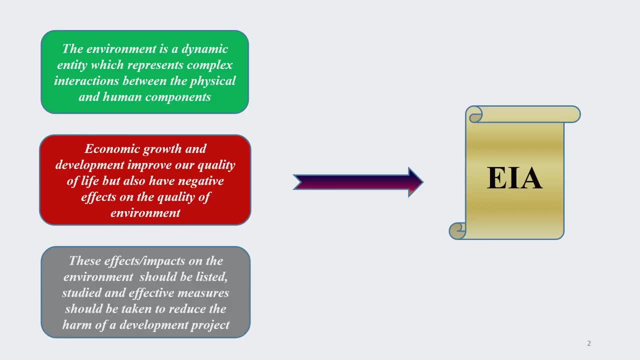 assessment. Now, what is actually EIA A? We know that environment is a dynamic entity, means which keeps on changing with time. Environment represents complex interaction between the physical and human components. We also know that economic growth and development improve our quality of life, but also have negative. 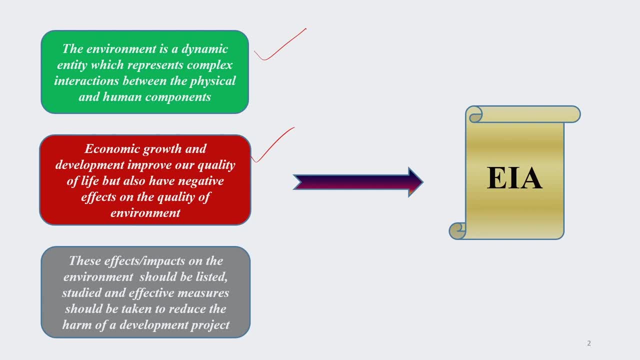 effects on the quality of our environment and we have discussed in great detail in previous lectures These effects of you know, various activities on environment. these effects or impacts on the environment should be listed, should be studied seriously and effective measures should be taken to reduce the harm of a development project. We cannot continue. 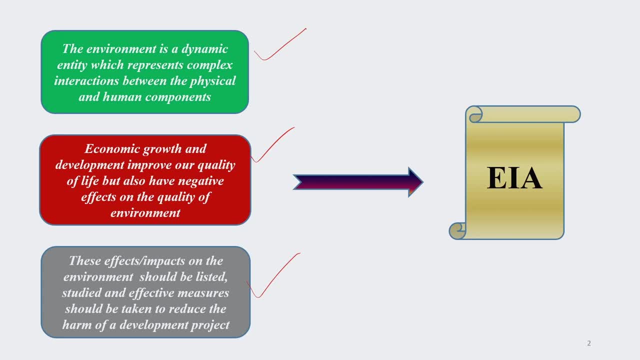 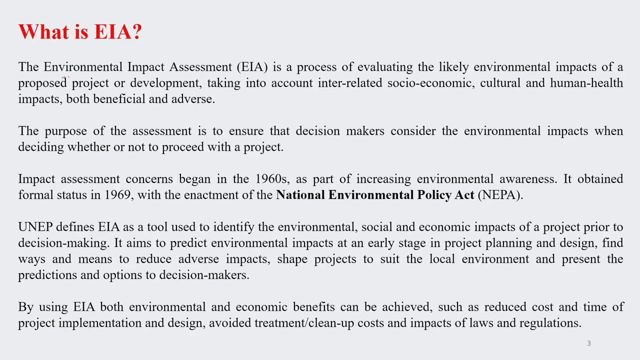 with our project activities without evaluating the environment. So all those things that terminate our project are not important. We can continue with things that terminate our, mentioned on the left hand side of your screen, basically gets taken care by environment impact assessment, EIA. it is a process of evaluating the likely impacts on environment by different 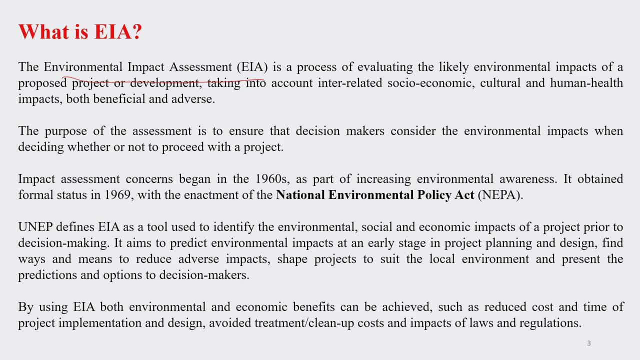 project activities, development activities, and which also takes into account the interrelated socio-economic, cultural, human health impacts and various other, you know, interactions which in a way, impacts the environment. The purpose of this assessment is to ensure that decision makers consider the environmental impacts whenever they decide whether or not to go. 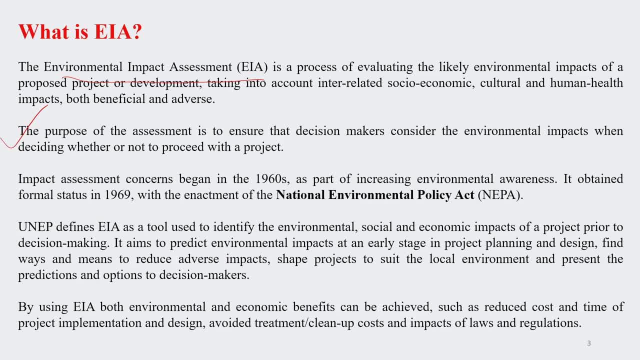 ahead with a project. That means, before the project is implemented in any location or site, it is important that you carry out an EIA of that particular project. Impact assessment concerns actually started around 1960s and this was as a part of increasing 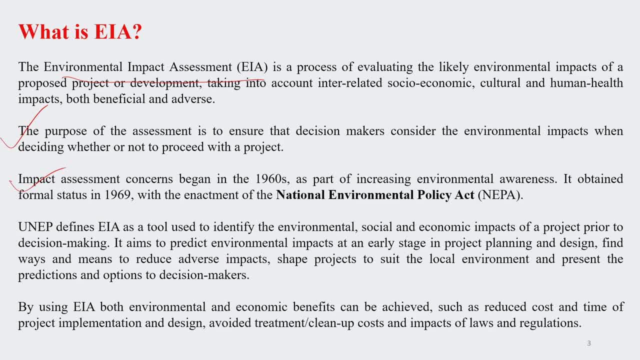 environmental awareness among society, among people. This EIA obtained the formal status only in 1969, with the enactment of National Environmental Policy Act, which famously known as NEPA. United Nations Environment Programme defines EIA as a tool which is used to identify the environmental, social and economic impacts of a project prior to decision. 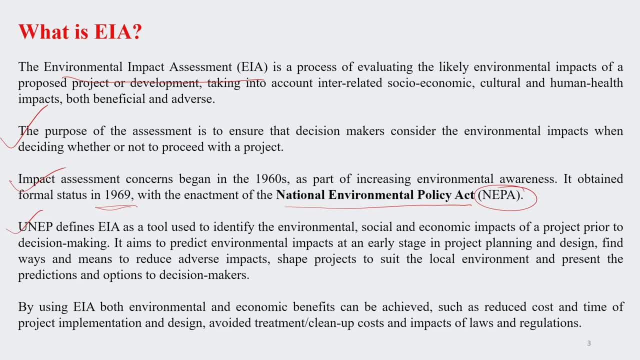 making, And this also aims to predict the environmental impacts at an very early stage of a project planning and design. It also finds the ways and means to reduce the adverse impact a project on the environment and also helps the project to adjust or suit the local environment. 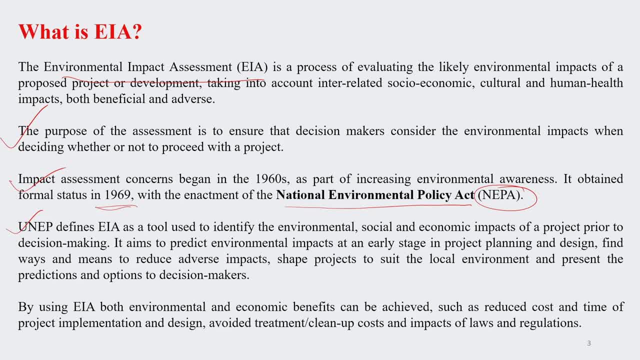 and thus present predictions and options to the decision makers. So you can understand that EIA, how important role is played by EIA for restoring our environment in one hand. on the other hand, also take the benefits of the natural resources for our sustainable development. 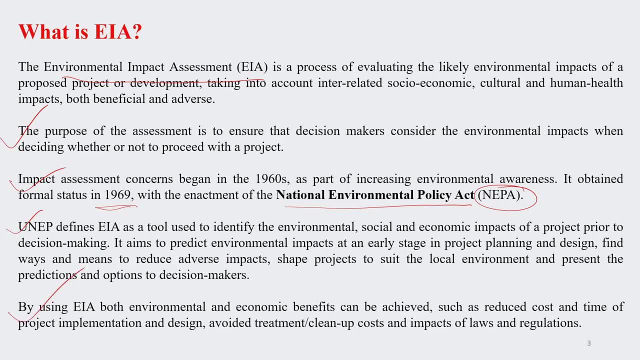 By utilizing environment. both environmental and economic benefits can be achieved how, such as reduced cost and time of project implementation and design, avoid treatment and clean up cost and also impacts of laws and regulation. So, essentially, if you carry out a EIA before the implementation of a project, you basically 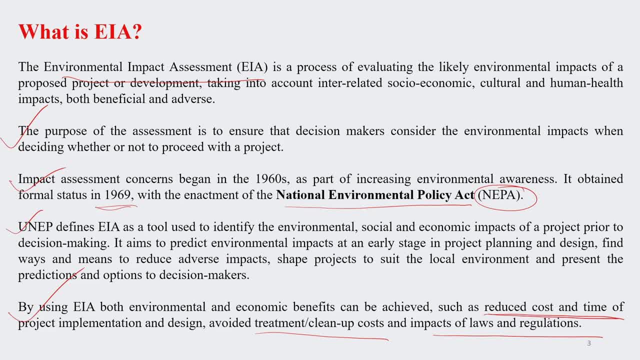 can avoid this kind of negative expenditures, Which means Not only cost your extra money, but also cost our environment. It also brings in certain, you know, litigation also. So why to go for this kind of negative aspects when we know that EIA is there and it is a? 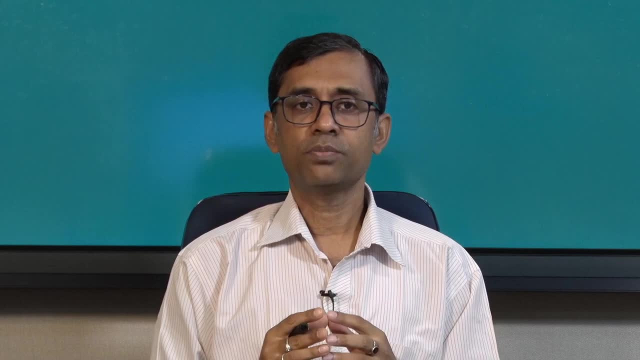 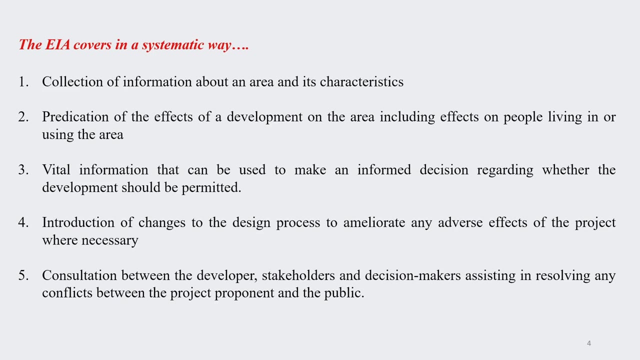 powerful tool to help us. So in this premise, the importance of EIA came into picture and today almost every project has to go through this particular exercise предpondering to the broader public. it is an integral part of EIA, which are the key. 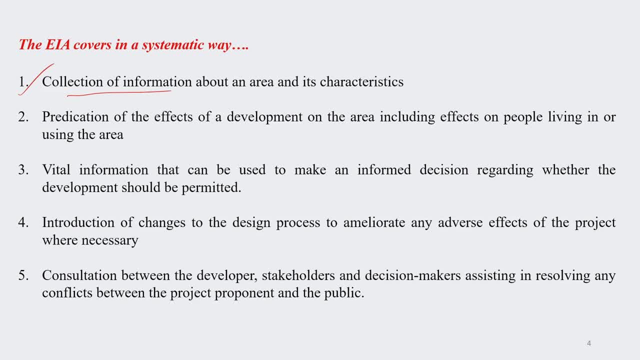 pillars of the social and environmental development and development where it covers certain, you know, important aspect in a very systematic manner. It helps in collections of information about an area and its characteristics, because if we do not know the area where the project is going to takes place and also what kind, 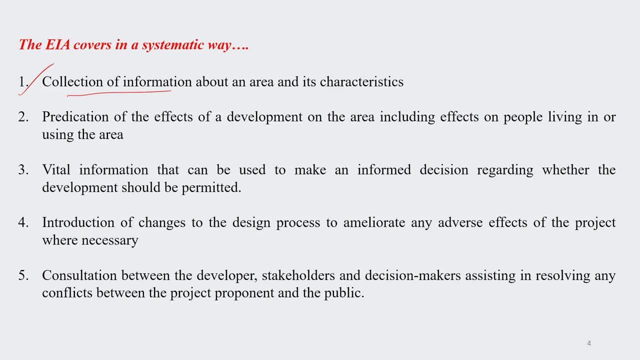 of flora, what kind of fauna, what kind of soil or what kind of that micro environment. I mentioned in previous slide that it helps in prediction of the effects of any development activity on the area, including the effects on people living in a or using that area. 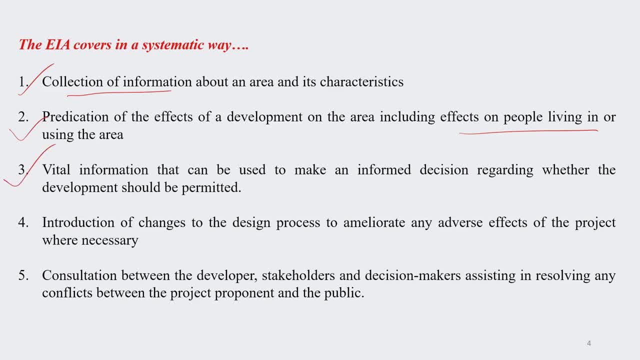 EIA also provides vital information that can be used to make an informed decision. This is very, very important for such kind of activity. You need to make an informed decision regarding whether the development that you are actually thinking is going to help people, whether it also will take care of environment. Because if you only go for development and on the 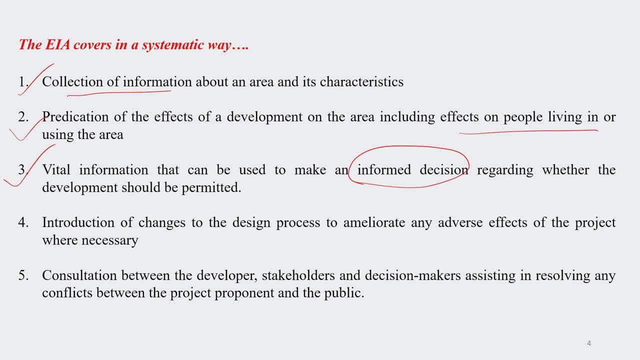 other hand, if your environment goes down, then actually you don't win this particular initiative. So your development, you are going up, but environment is going down. So basically we lost. So the best part is that how to do this. So the best part is that how to do this. 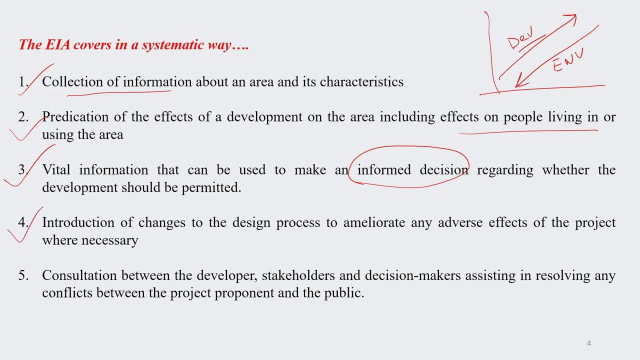 to find out a balance and EIA helps you to decide. It also helps in introducing the changes in the design processes when you plan the project and to ameliorate any adverse kind of effects of the proposed project on the environment. So, as I said, that it helps like. 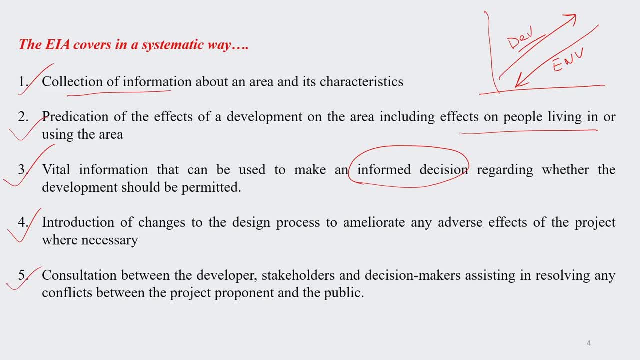 a kind of an early warning. EIA also promotes, facilitates consultant consultation between developer, various stakeholders, decision makers, the users for whom actually everything is being done in resolving any kind of conflict between the project proponent and the public, Because if this is taken care of at the very beginning, then you can actually avoid complicated. 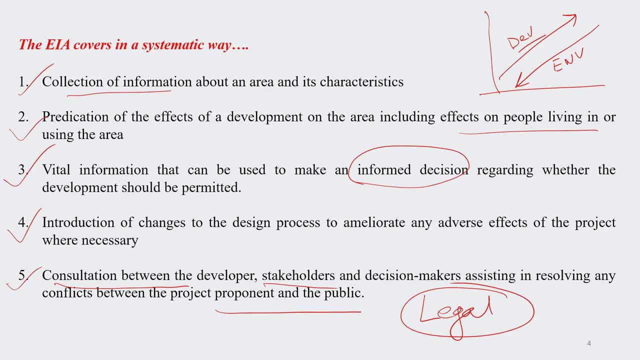 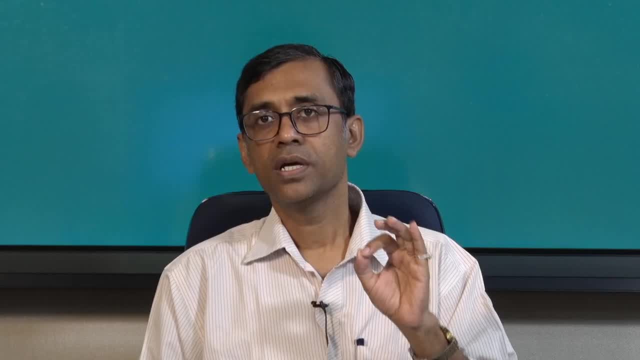 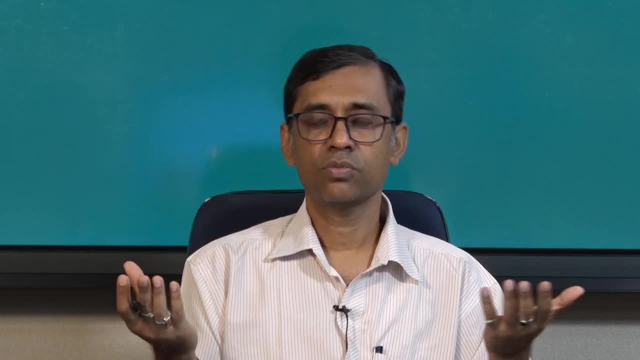 legalities which may actually, you know, push your project backward. You may not even think that you are able to start. even So, the relevance of a particular project, if it gets postponed by a month or six months a year, you understand, the relevance of that project is almost lost. 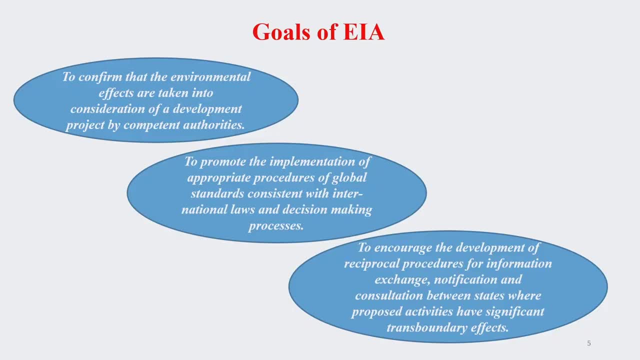 Now, goals of EIA. What are the different goals? It helps to confirm that environmental effects are taken into consideration of a development project by the competent authorities. These competent authorities are the people who are responsible for the development of the project. They are the people who are responsible for the development of the project. They are the people who are responsible for the development of the project. They are the envoys for the development of the project. They are the people who are responsible for the development of the project. They的人inful, do all the work they need to the這個. 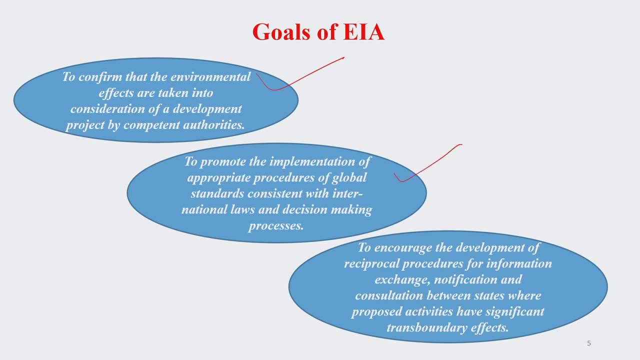 could be private as well as government entities. This also promote the implementation of appropriate procedures of international standard which are consistent with laws, international laws and decision making processes. Today, India is a country we cannot play in isolation. Any product or development that we plan to do, it has to be of world standard. 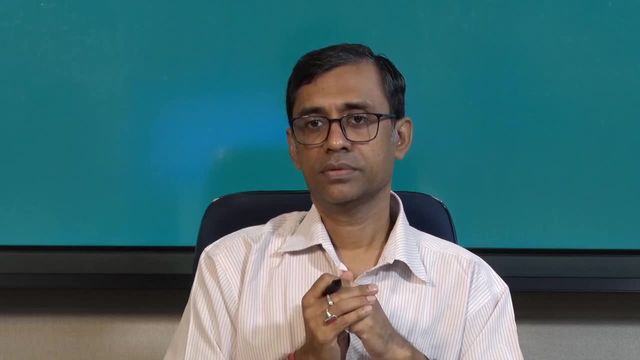 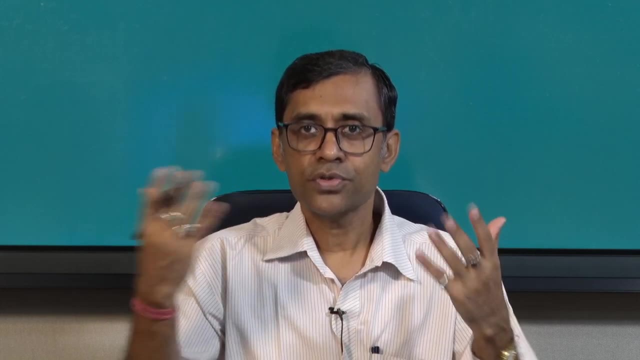 Then only our product is played in the world. puisquising ability- The development is done by international standards, not between the companies Due to this terms as an example, will have a market. Unless we have a market, then producing more and more will not fetch. 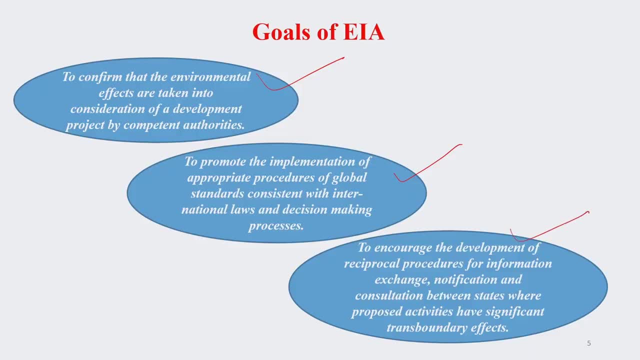 us anything. GIA also encourage the development of reciprocal procedures for information exchange. Suppose, in some project you are going to implement and there are couple of stakeholders who are also involved in this exercise or in that area where actually you are going to start, they may seek some information. So there has to be a kind of a reciprocity between project. 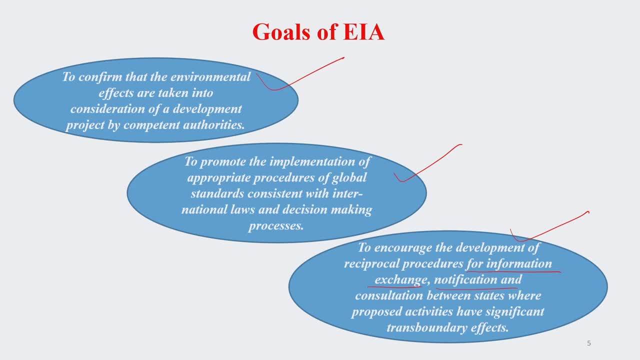 proponent and also the other stakeholders. Notification and consultation between states where proposed activities have significant transboundary effects needs to be taken care of. Suppose you know there are two states, all right. Suppose this is one state A and this is one state B. 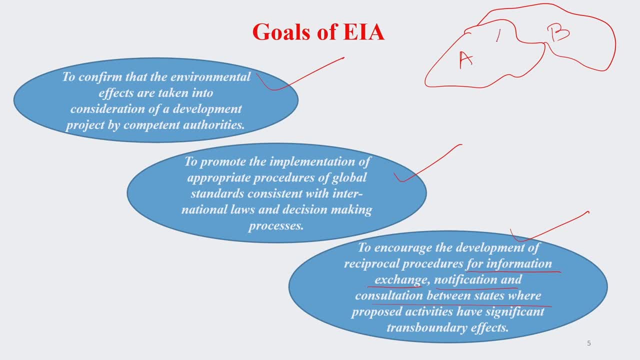 Now you have a project which actually has the boundary or right at the. perhaps half of that project is in this state and half goes into other state. It could be a watershed project, it could be anything. So in such condition it is important that the project proponent, if 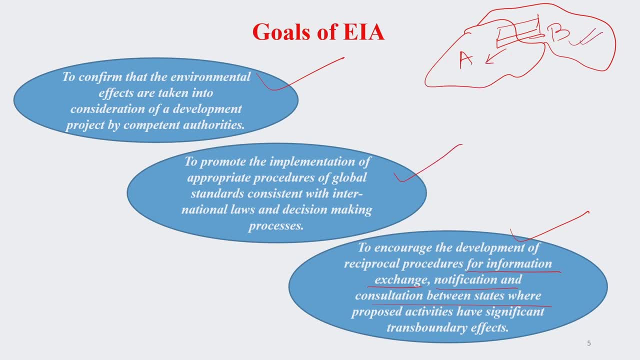 is this state must talk with state B as well, the bordering state. The key is dialogue. So through dialogue you actually, at the before the implementation of the project, you address all the issues that could prop up otherwise in future and that will delay or stop your. 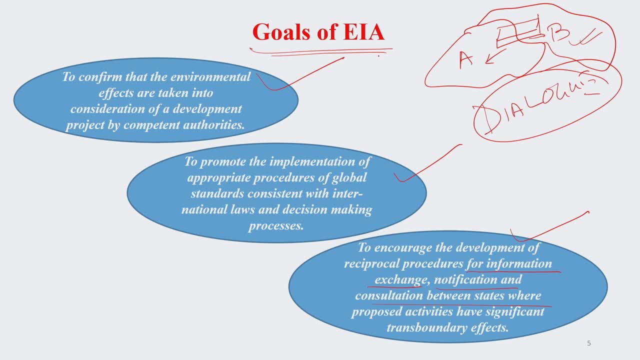 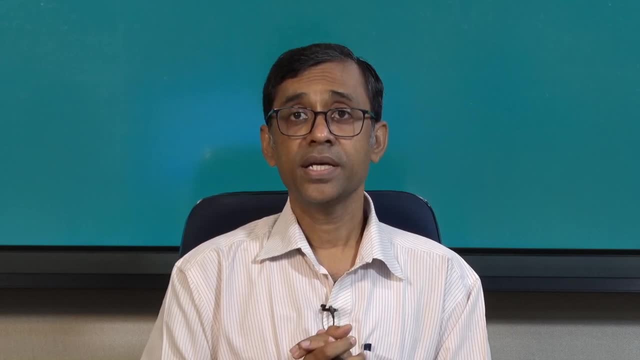 project. So these are the goals of EIA Basically, as you understand, EIA is not to stop any project. rather, EIA, you know, protects your project from various unwanted expeditious decisions. So these are the three goals of EIA. basically, as you understand, EIA is not to stop any. 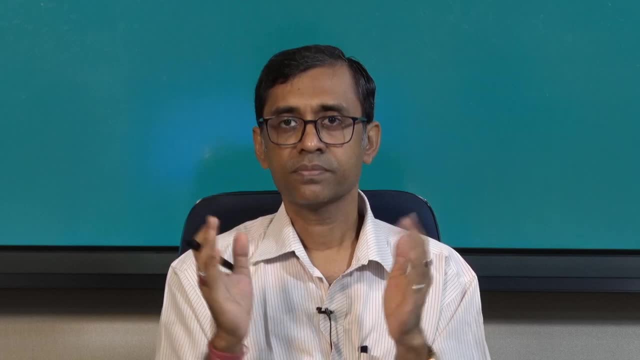 project. Rather EIA, you know, protects your project from various unwanted expenditures, so you can do the work. that should not happen if you do not stop it. These are some of the expenditure: unwanted threats, legalities, etcetera. okay, 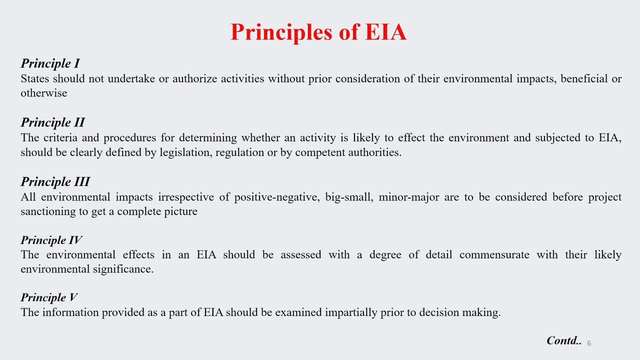 Now let us know about the principles of EIA. Like any other- you know, tools or any other approaches- EIA also follows certain principles. First, states should not undertake or authorize activities without prior consideration of their environmental impact, beneficial or otherwise whatever, whether negative or positive impact. but it must be considered before the 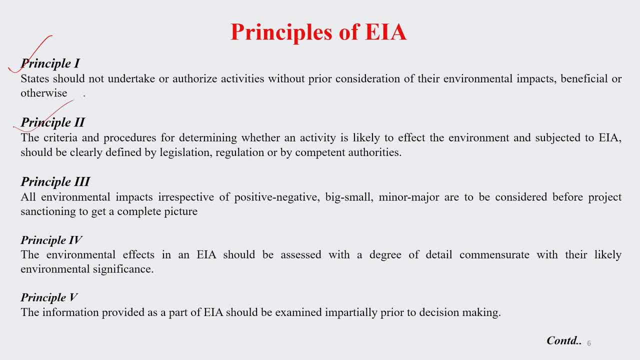 project has been undertaken. Principle number 2, the criteria and the procedures for determining whether an activity is going to affect your environment. that has to be seen through EIA and it should be clearly defined by legislation, regulation by competent authorities. Again, this is not to stop your project, but to give your project a kind of a safety. 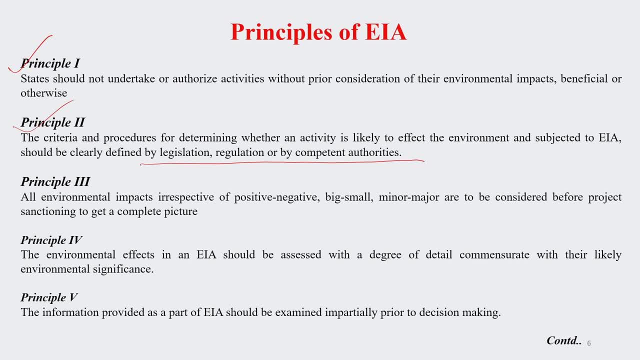 net which otherwise, in future, you might face something which can totally, you know, jeopardize your project. Principle number 3, all environmental impacts, irrespective of positive or negative, big or small, minor or major, has to be considered before project sanctioning. to get a complete 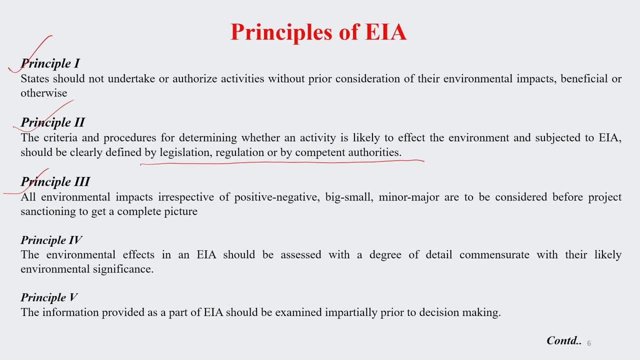 picture. You cannot do this, carry out this exercise once you actually sanction the project or implement it. there is no use. In certain cases, you may have certain example that EIA and the implementation is going side by side. No, ideally that should not happen. 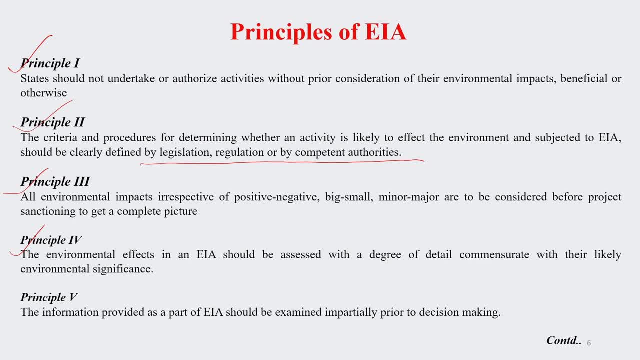 Principle number 4, the environmental effects in an EIA should be assessed with a degree of detail commensurate with their likely environmental impact. Thank you, Or significance. Number 5, the information which are provided as a part of EIA should be examined impartially. 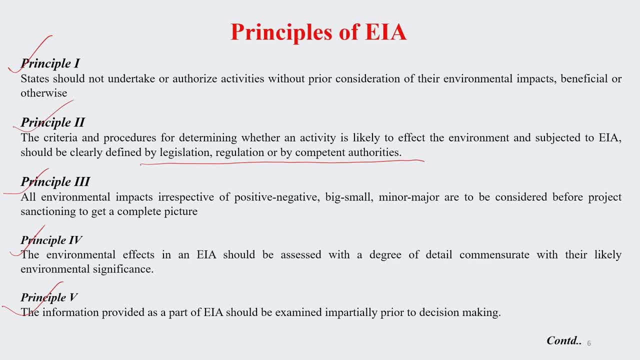 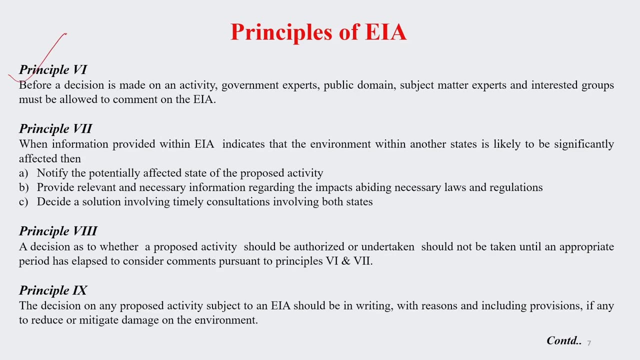 prior to the decision making. So, friends, as you see that the benefit of EIA will only be achievable if you do it prior to implement, prior to taking the decision, prior to the sanction of the project. Number 6 principle: before a decision is made on: 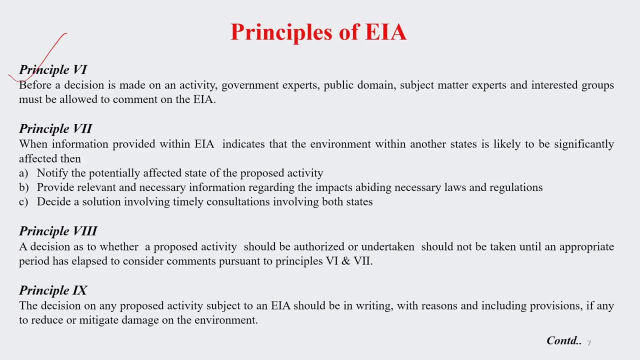 an activity, government experts, public domain subject matter experts, interested groups, potential beneficiaries. they must be allowed to comment on the EIA exercise that is being carried out. In a sense, this exercise has to be taken in a very democratic manner. There should 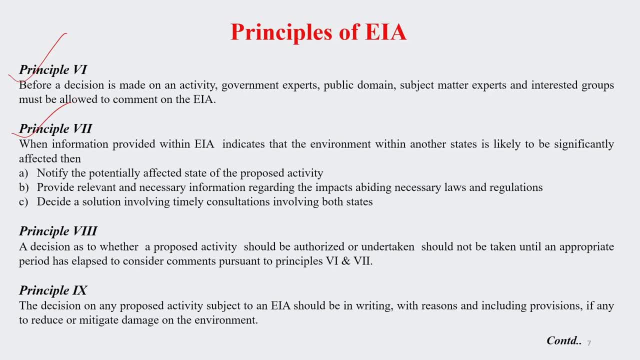 be considerable amount of transparency. Principle number 7,: when information is provided within EIA, it indicates that there is a need to ensure that the environment within another state is likely to be significantly affected. Then what should we do? a We should notify the potential affected state of the proposed activity. Often there, 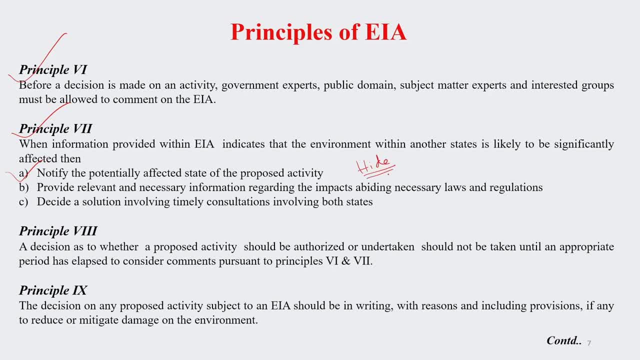 is a tendency to hide it. we should never do it. So notify the potential effect to the neighbouring states. Provide relevant and necessary information regarding the impacts which are avoiding necessary laws and regulations. Thank you, and regulation. decide a solution involving timely consultations involving not only the state that 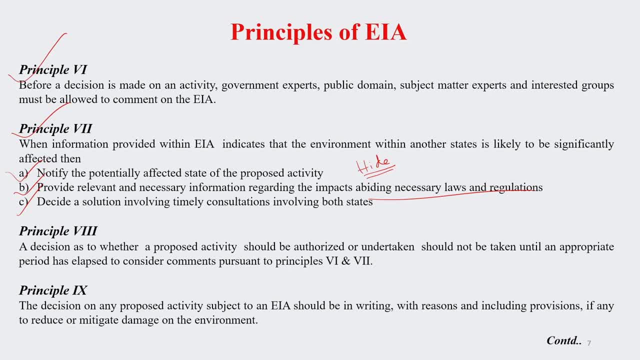 you are implementing, but both the states or the states, whichever is affected by the potentially going to be affected by the project number eight: a decision as to whether a proposed activity of your project should be authorized or undertaken must not be taken until an appropriate period has crossed to consider the comments pursuant to principle six and seven. so in a sense, you must not. 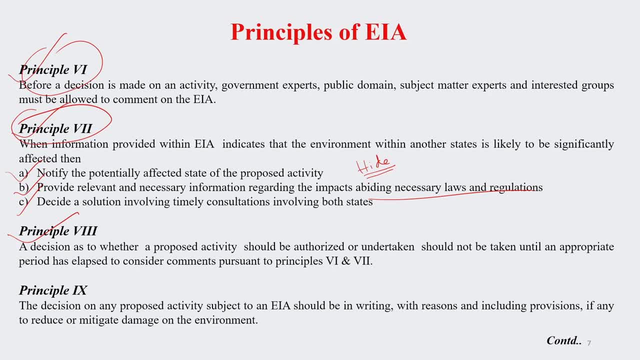 hurry it up, give some significant amount of time to the people, to the neighboring states, to study the eia report or outcome and give comment. then you take a decision. number nine: the decision on any proposed activity subject to eia should be in writing. no verbal communication is encouraged because that does not have any record. so with 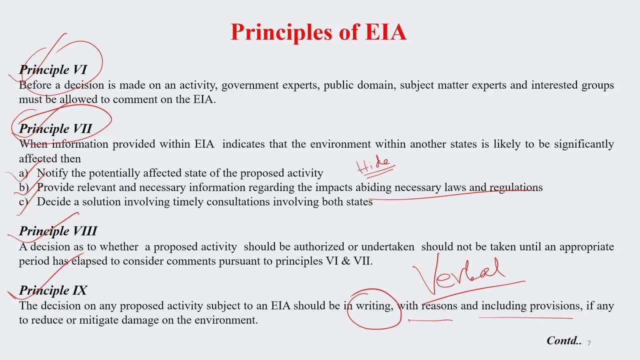 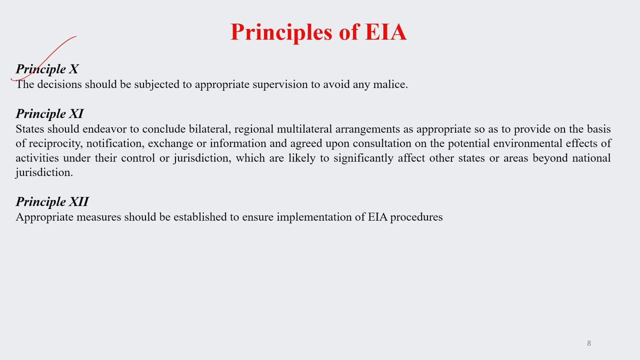 regions and including provisions if anyone to reduce or mitigate the damage on the environment has to be given in written form. okay, number two: you also have to give full consideration to every zw arranged in any case. at least enough reason only: equal distribution within an action that helps you to approachevents and 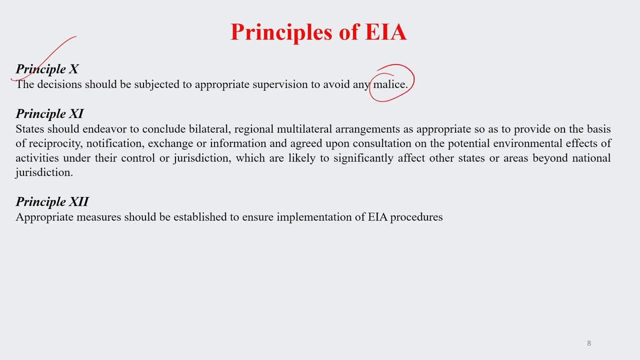 you have to maintain that if, but it should be taken seriously for the functionality use of competence. esseble out to be a good example and take all the possible proper Aboriginal practices and rituals. now tell us seriously whether, in schools, how to crunchy experience, change yourself, is it? 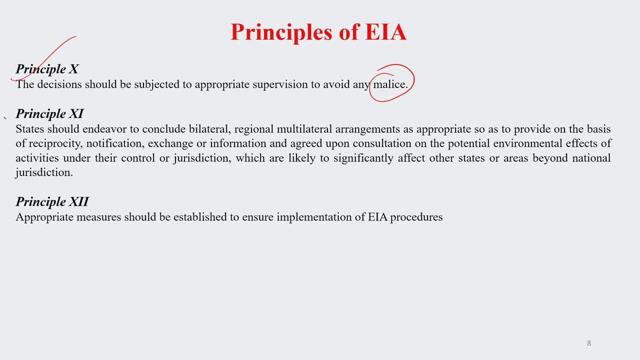 right or not is state that how one should actually follow the EI activity Number 11, the states, the involved states, must, should endure to conclude bilateral, regional, multilateral arrangements as appropriate, so as to provide, on the basis of reciprocity. 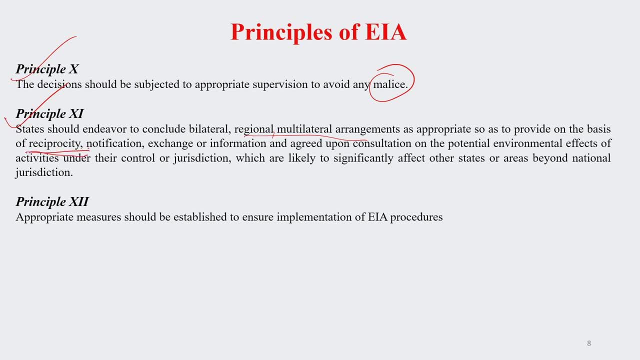 This is very important: reciprocity: Things should be notified in advance, exchange of information, and one should agree for consultation on the potential environmental effects of any activity under the proposed project. The last principle, number 12,: appropriate measures should be established to ensure implementation. 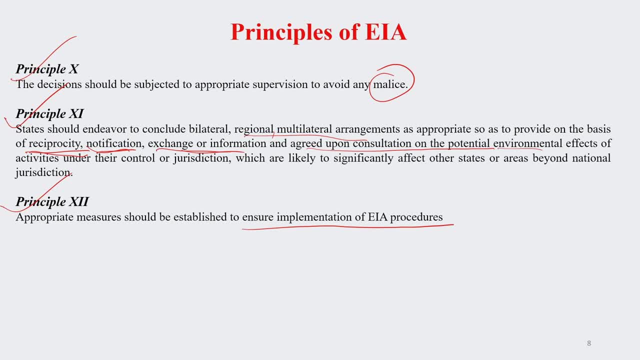 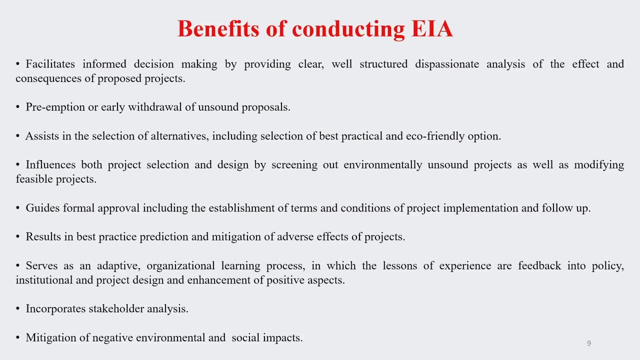 of EIA procedures. We have all those things in paper, but unless until this is implemented in a stringent manner, then the purpose of having these principles, the rules, regulations system, has no meaning. Benefits: why do we actually do EIA? There has to be some benefits, right. and what are? 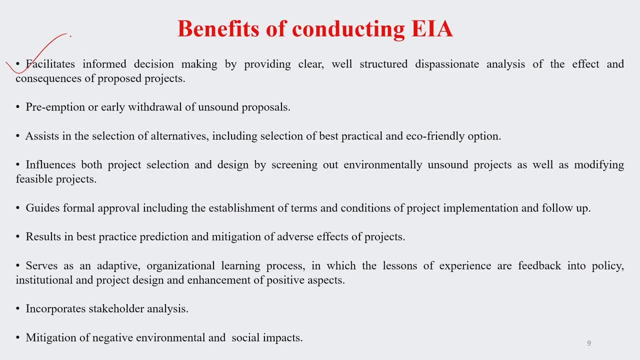 those. It facilitates informed decision making by providing, you know, clear card information, analysis of the effect of various activities and consequences of the project. It gives a kind of a predictions or opportunities for early withdrawal of unsound propositions. Thank you. proposals or activity: If there are certain activity which has a negative impact, if you 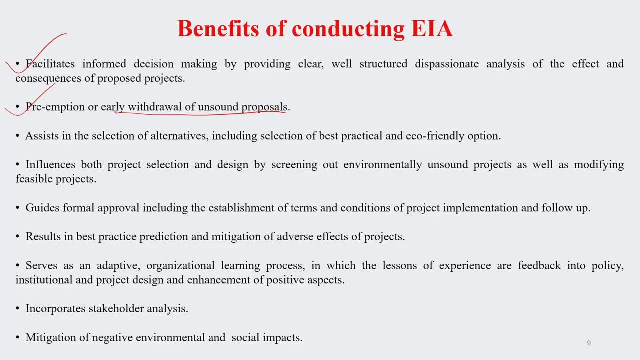 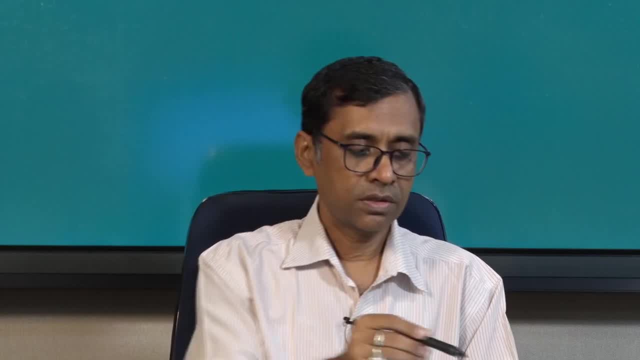 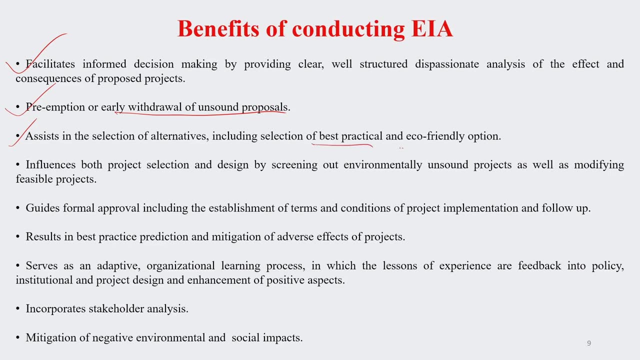 are able to see it from the EIA exercise, then why should you go for that? and if you go for that, then one has to be ready also to face the consequences. EIA also assist us in the selection of alternatives, including the best practical and eco-friendly. 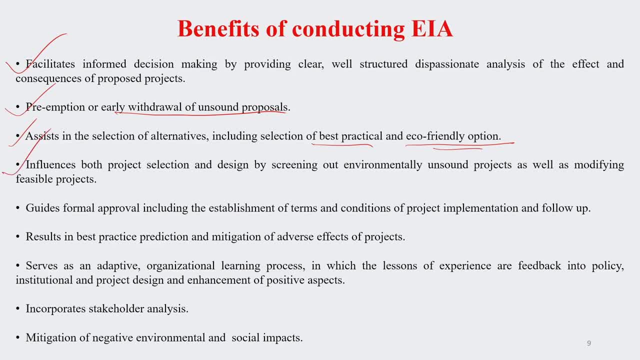 option. EIA also influences both project sanction and design by screening out environmentally unsound project as well as modifying feasible projects. So if you have certain you know proposals for two or three projects, EIA will help you to identify the projects which are going to impact your environment, so remove them. EIA guides formal approval, including: 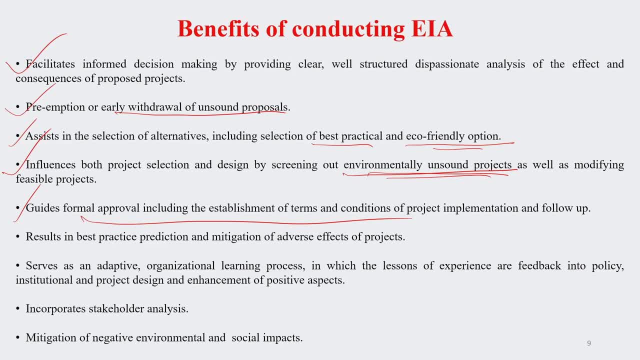 the establishment of terms and conditions Of implementation of project and then follow up. It also results in best practice prediction and mitigation of adverse effect of the project. This also serves as an adaptive organizational learning process in which the lessons of experience are feedback into your policies institutionals. 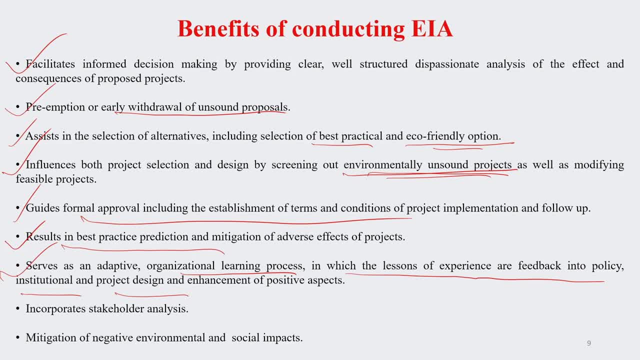 or project design, or also in enhancement of positive aspects. So essentially, it helps you to develop an adaptive system which can actually adjust with certain changes in the system. It also incorporates stakeholder analysis. very, very important, very important. because you know that before any project, especially the project, 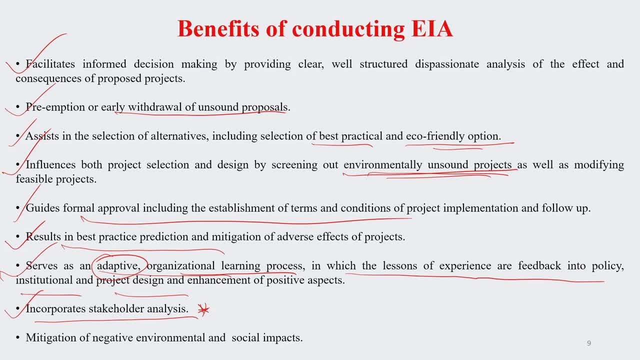 which is going to utilize natural resources of an area, EIA is must and stakeholder analysis or discussions, Which actually EIA gives you the opportunity, is one of the best thing. Then mitigation of negative environmental and social impact: This is also is another important benefits. 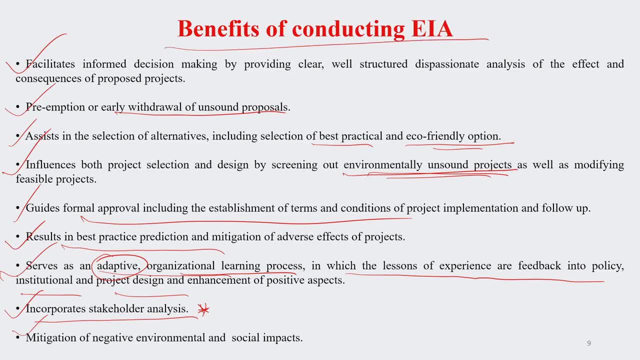 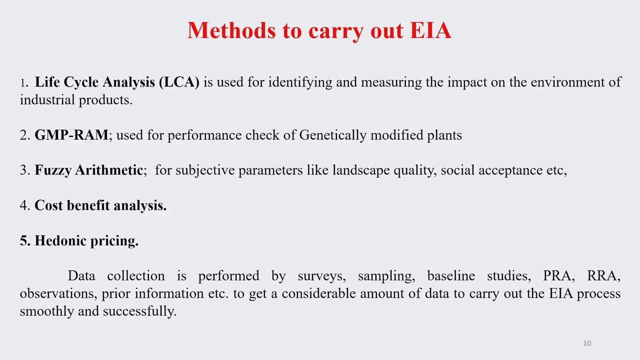 of conducting EIA in an area where you are going to propose a project. Now let us see the methods which actually we use to carry out EIA. There are various methods. I will go one by one. Certainly in this one Lecture it will not be over, So I will follow it up with upcoming lectures. So what are? 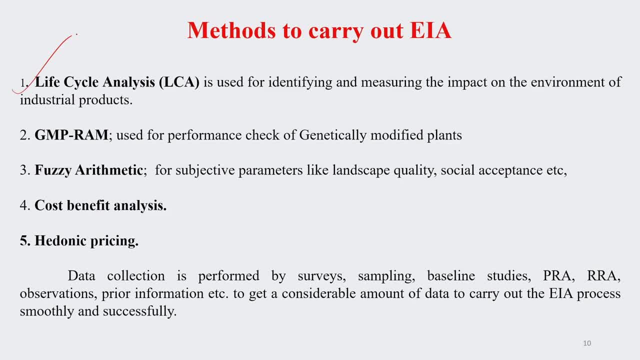 the methods. The first life scale analysis, LCA. I am sure most of you might be knowing about LCA. Some of you are professional, may be using it also. LCA is used for identifying and measuring the impact of any activity on the environment. GMP RAM. this is used for 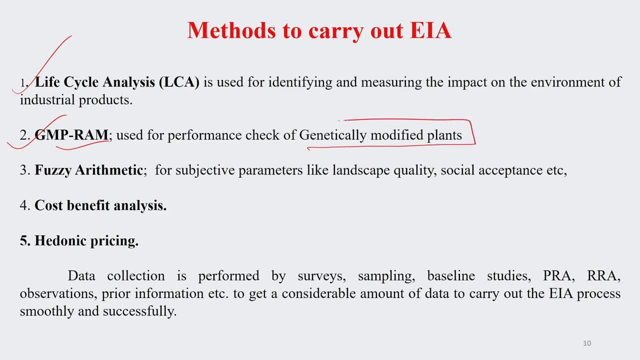 performance check of genetically modified organisms. This is used for the process of genetic modification. This is used for genetic modification. This is used for genetic modification modified plants, GMO. it is a hot topic. right in the last 10 years. we have heard lot of 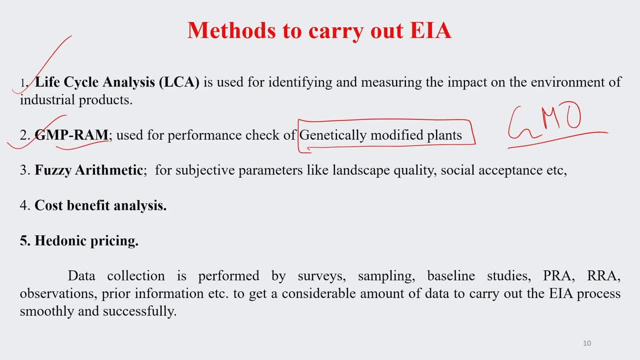 you know, deliberations nationally, regionally, internationally about genetically modified organisms, plant is one of that Fuzzy arithmetic. these are actually method for subjective parameters like landscape quality. social acceptance means you are going for a project whether that project is socially accepted by the peoples residing there. so those kind of analysis, fuzzy arithmetic method. 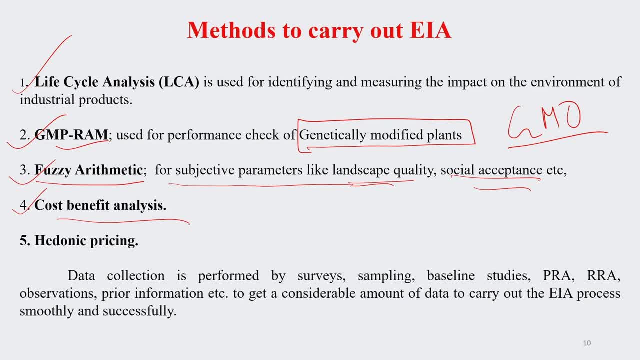 will help you Cost benefit analysis. you know that for that project, how much you are going to spend and how much you will going to earn, and also ecological cost benefit. you need to also analyze Hedonic pricing. this also helps to find out the impact of an project on the environment. 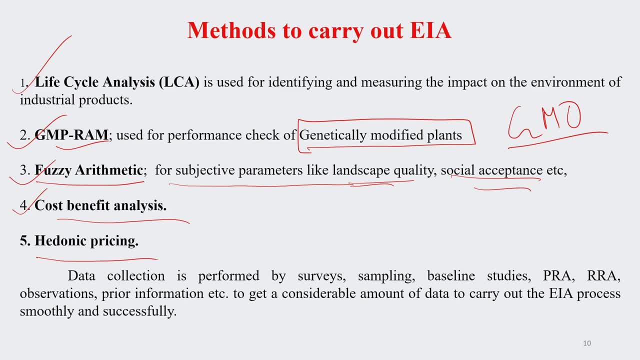 The data collections in EIA method largely performed by surveys, sampling, baseline studies and PRA, RRA. I hope you recall that at few you know lectures back we have discussed in great detail about participatory rural appraisal and rapid rural appraisal. So these all are the you know exercises or tools which actually can be used for carrying 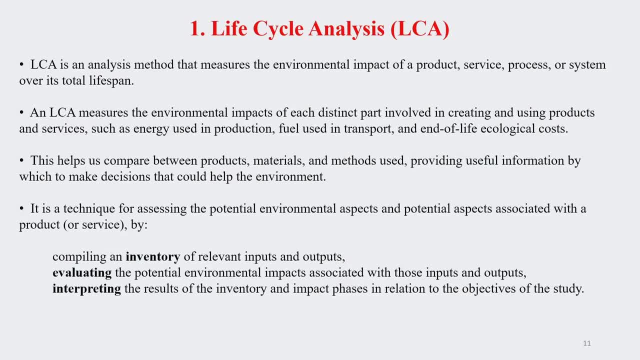 out a successful EIA. So the first method is life cycle analysis. Now, LCA is an analysis method that measures the environmental impact of a product or service, process or system in total life span in area, and LCA measures the environmental impact of each distinct part that is involved in creating and using the products and services. 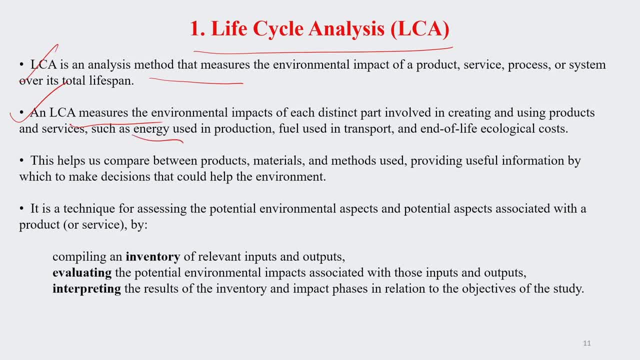 So, for example, energy used in production, fuel used for transportation and end of life ecological cost. that all we should not forget When we calculate the cost of fuel, energy, we must also learn to calculate, learn to value the ecosystem, services or the ecology or environment. 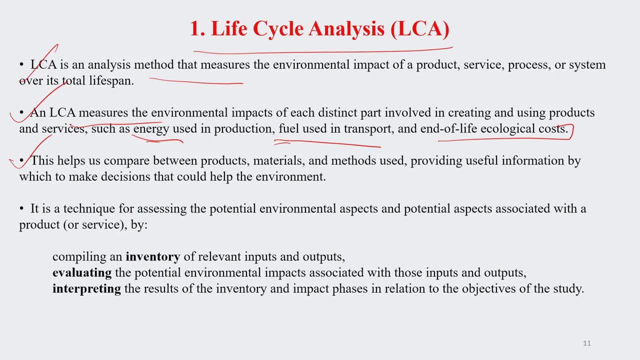 LCA also help us to compare between products, materials and services. Materials, methods which are used and which are utilized for providing useful information through which we can actually make decision and, finally, which could help to keep our environment intact. Life cycle analysis is a technique for assessing the potential environmental aspects and potential. 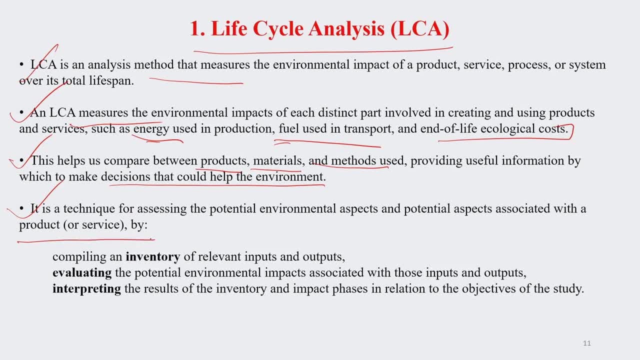 aspects which are associated with a product or service By compiling an inventory of relevant inputs and outputs, evaluating the potential environmental impacts associated with those inputs and outputs, interpreting the results of the inventory and impact phases in relation to the objectives of your study. So, as you see that LCA basically help you to get a picture of the entire sphere of the 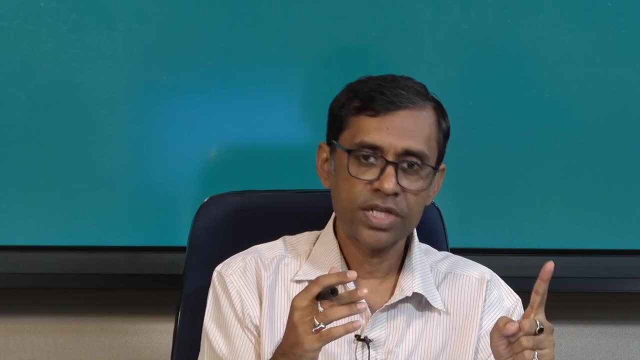 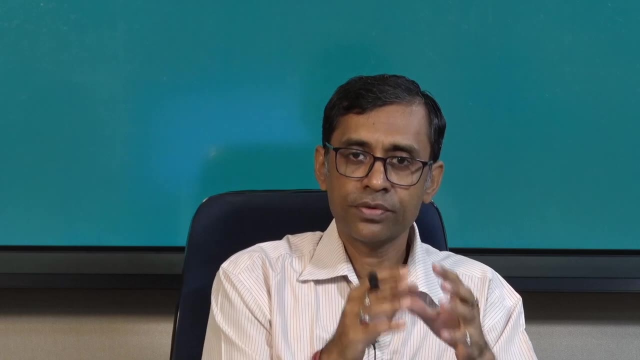 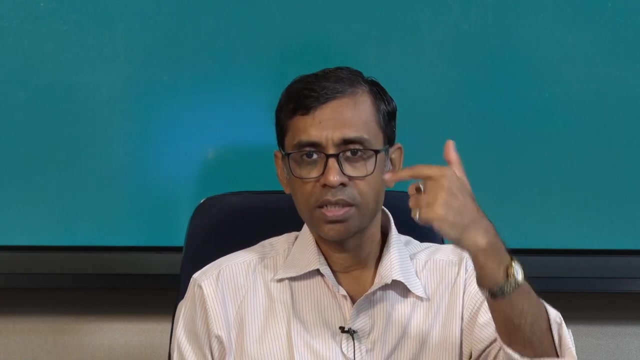 environment, That sphere of the impacts of an project in a particular area. It looks not only in a particular point of time how it impacts, but it also looks at for a you know longer time span, throughout the you know life of that project, how it is going. 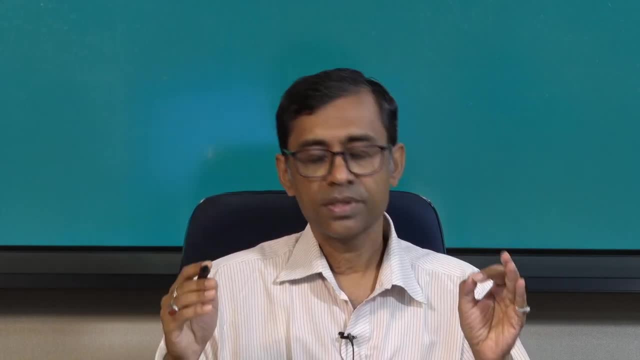 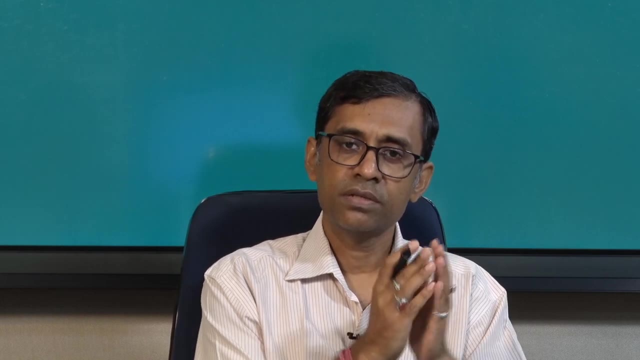 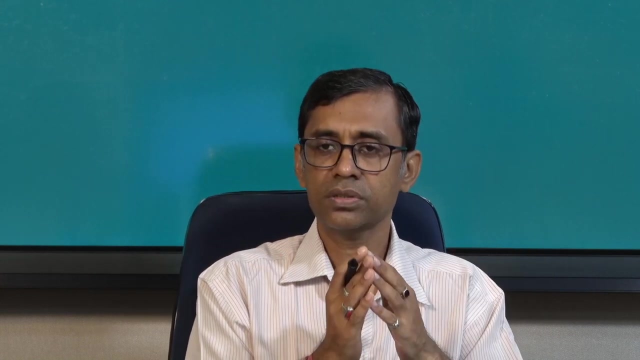 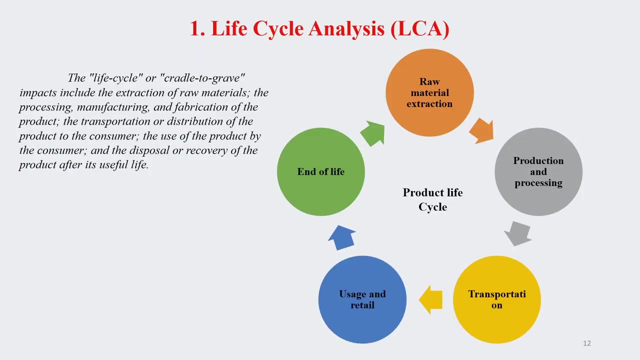 to impact the environment and this gives a reasonably good idea to the decision makers that how a particular project implementation is going to impact the environment, the natural resources and the society altogether. In LCA there are few stages. People call it life cycle or cradle to. 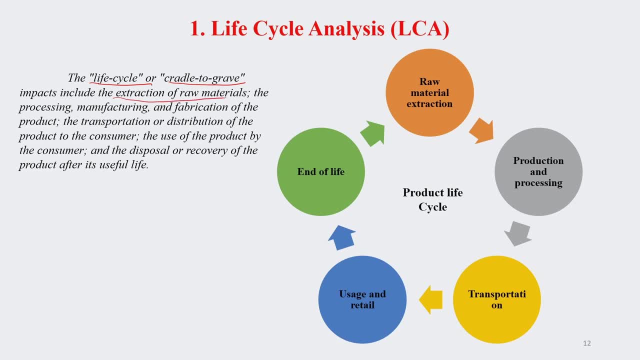 grave. These impacts include extraction of raw materials, then production and processing. So when we say raw material, these are largely natural resources. I hope all of you understand that. So once you extract, then you go for production and processing And during this, 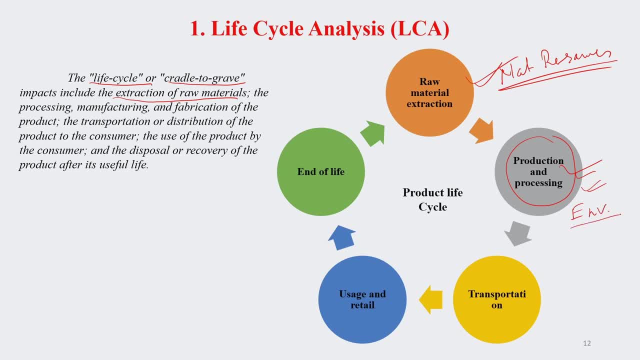 process, there is a chance that you are going to impact the environment, So this particular phase need to be looked at very carefully. Transportation: once the product is developed, certainly you need to transport from production site to the you know delivery site. Then it goes finally to users or retail shops where your product will.